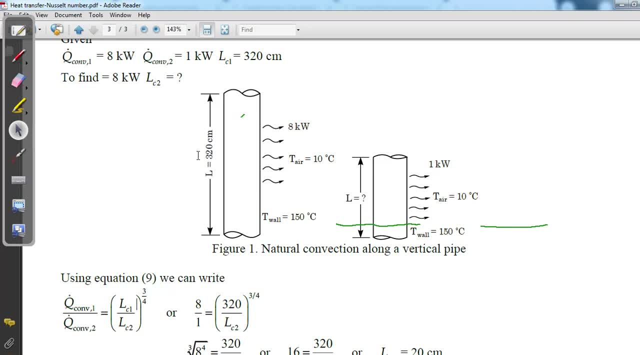 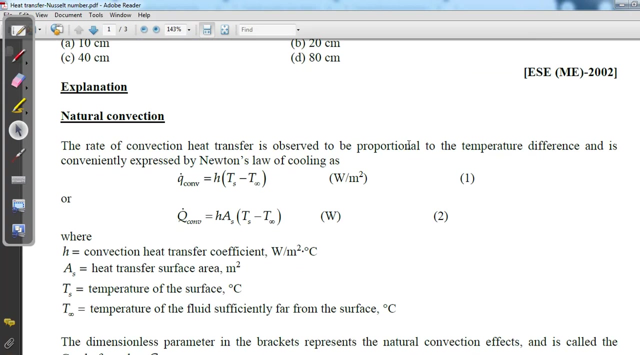 So this is the diagram. First, it is saying that the length of the pipe is 320 centimeter. Some hot fluid will be flowing in the pipe. Because of that, temperature will rise of the surface around 150 degree centigrade and outside temperature is 10 degree centigrade. So definitely that heat will be flow from high temperature to low temperature at a rate of 8 kilowatt. So now it is saying that we don't need 8 kilowatt, We just need 1 kilowatt, Others conditions are remaining same. So what will be the length of the pipe? So this is the question. So now to solve this question, we have to study some vertical concept and some formula. 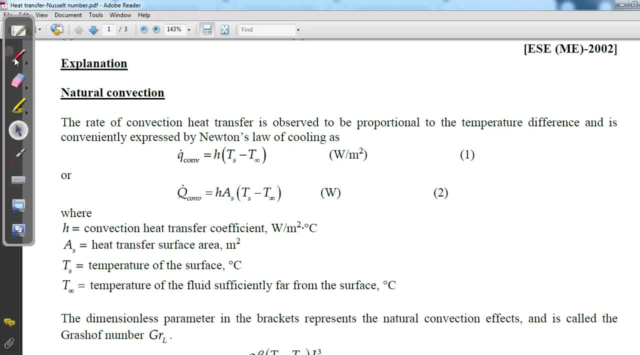 For that, let's study it. So it is saying natural convection. So for natural convection we will need this Newton's law of cooling which says: Q convection is given by H into A, S, T S minus J infinity. H is convective heat transfer coefficient, A S is heat transfer surface area, T S is temperature of the surface and T infinity is temperature of the fluid sufficiently far from the surface. So this is the formula. 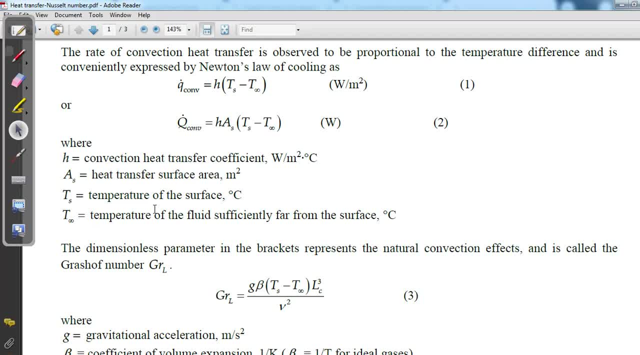 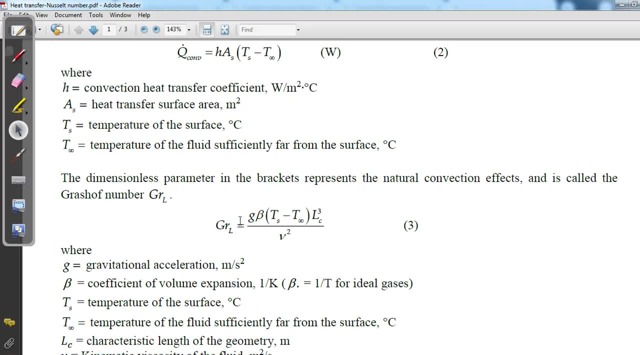 So we would be needing some dimensionless parameters in natural convection effects For that first number is defined Grashof number, Grashof number formula. right now to solve this question, we just need the formula. How it is coming we will see in the theoretical lecture. 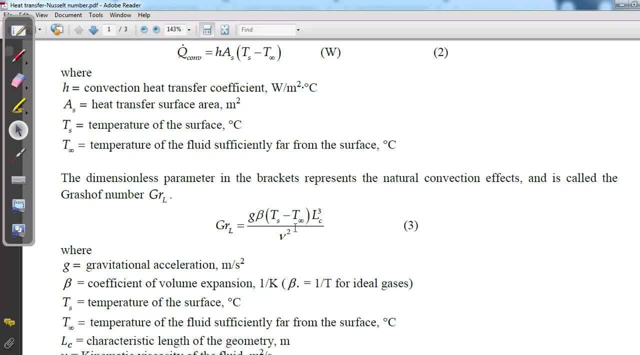 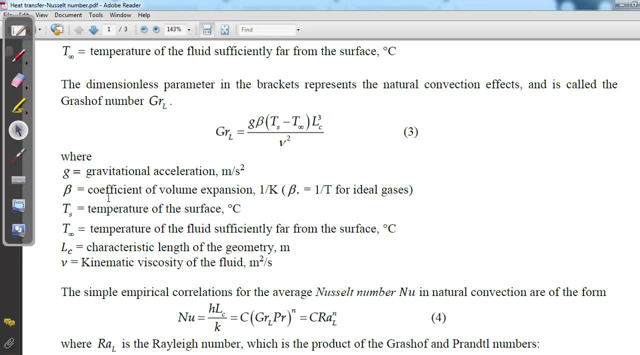 So Grashof number is given by G beta T, S minus T, infinity, nu, whole square L, C, Q to power Q. So these are the notation that G generates gravitational acceleration, coefficient of volume expansion, psd, infinity. you know lc is characteristic length of the geometry. 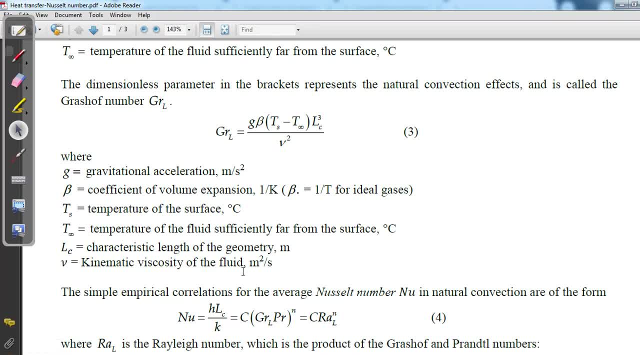 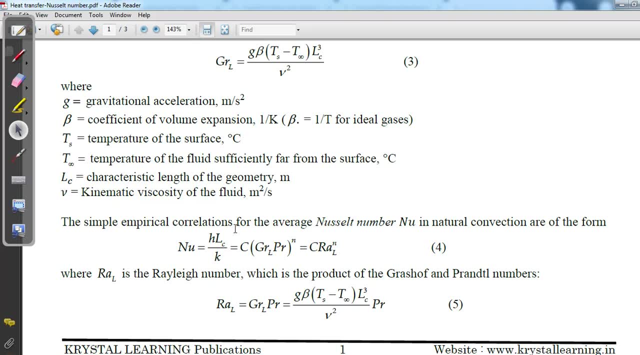 will depend on what type of geometry it is given. and k is kinematic viscosity of the fluid. again, another parameter, that is nusselt number, in natural convection is given by h, lc, by k that is equal to c, greshoff number into prendel number to the power n. okay, and that greshoff. 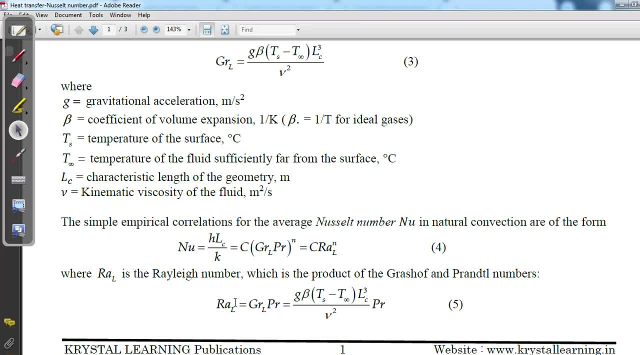 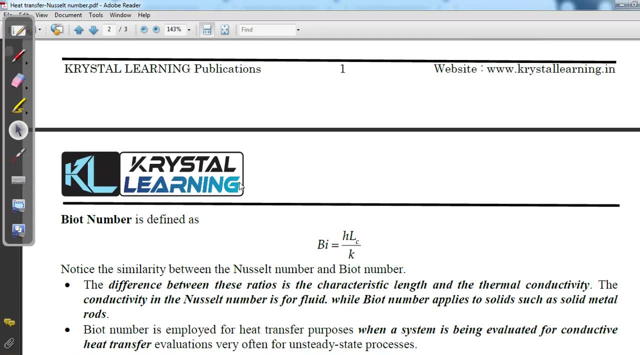 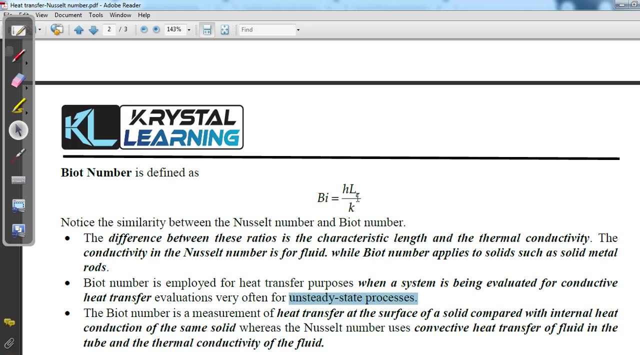 number and prendel number. product is known as rayleg number. so this rayleg number is given by this. so you see, nusselt number is given by h, lc, by k and in, and in another chapter of unsteady state processes or transient state condition, a number will come, biot number, given the same. 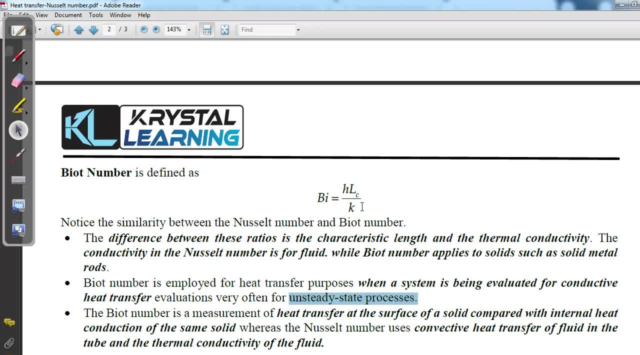 notation that is h lc by k. so in interview they always ask maximum time. they ask that what is the difference between biot number and nusselt number? because their formula notation is given by same, that is, h lc by k. so two basic difference is this: 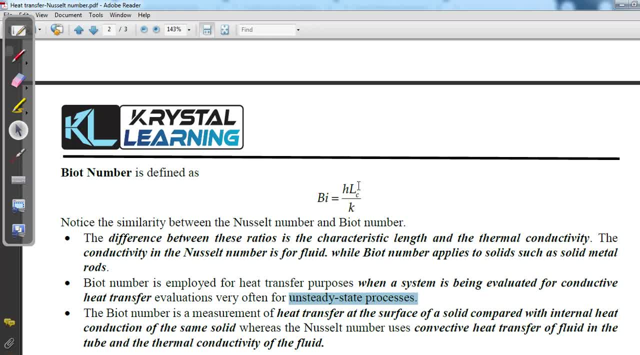 lc characteristic length. so in both of the, that is, nusselt number and biot number, lc will be different. calculation of lc will be different in both the cases. and this conductivity, thermal conductivity. so what is the difference? that thermal conductivity in nusselt number is taken. 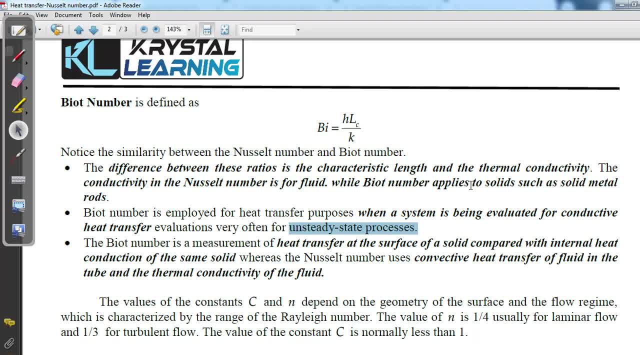 for fluid, while in biot number it applies to the solid, that what is the solid like solid metal. so this is the basic difference. so we won't be going to talk about the difference between biot number and nusselt number, going into much details, but just keep this question in mind, that 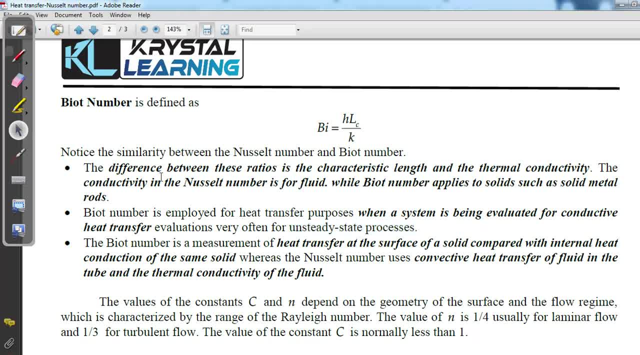 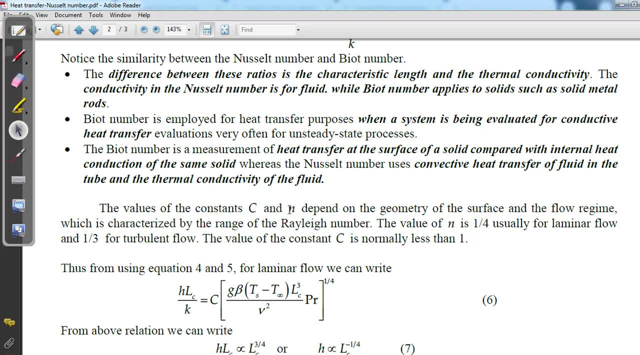 what difference between biot number and nusselt number. so, again in the previous formula, we have to know the value of constancy and n and, more importantly, we have to know the and and will depend on the geometry of the software. that. what is the geometry? and flow logic? that well. 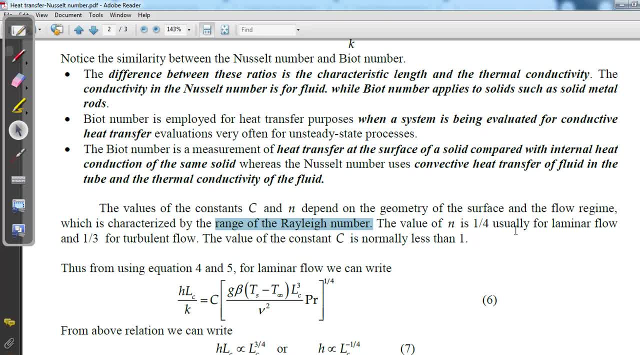 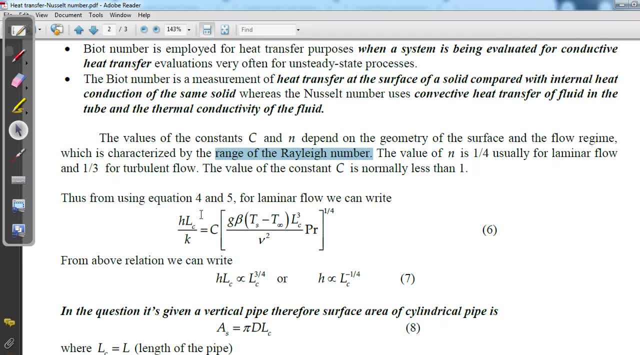 that flow you assume assume as laminar flow. so n we will be taking as 1 by 4, 1 divided by 4. so this is the nusselt number formula, that is, hlc by k, equal to c times gresham number into. 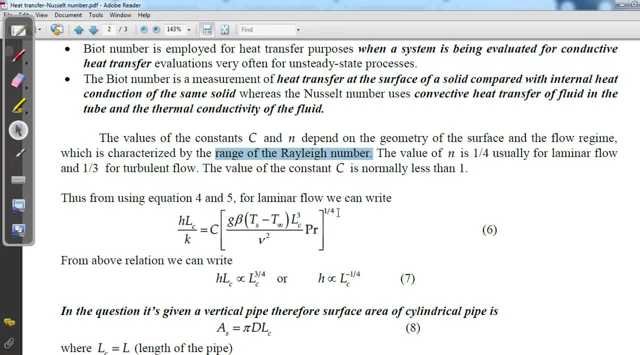 number to the power n, and we will and we would take as 1 by 4. so all these things are constant for this given question, that is, k, c, g, b, t, s, t, infinity, nu and prender number. so here we. from this equation we see that hlc is directly proportional to lc, to the power 3 by 4. now lc will 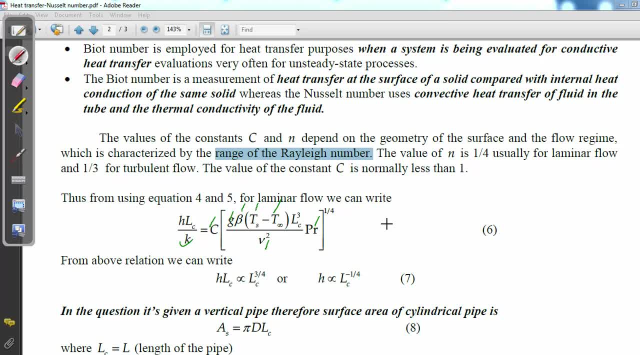 come on the on the on this side, and in division form. so it will be taking 3 by 4, minus of 1 when it will go upside, so it will come 3 minus 4 divided by 4 or minus 1 by 4. so here we got. 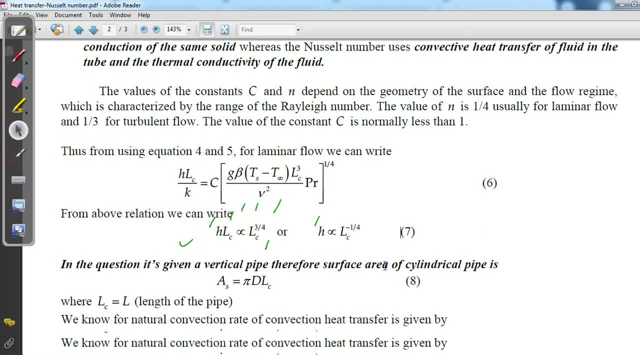 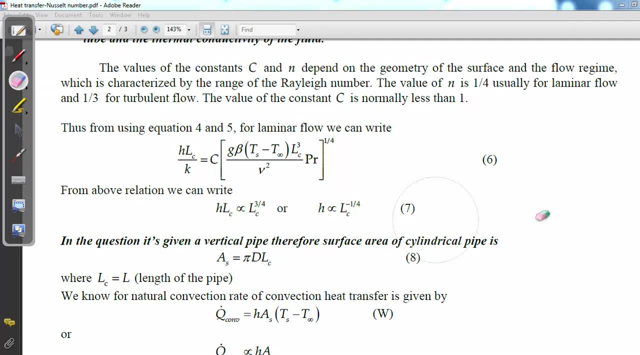 one relation, that is, heat transfer. convective heat transfer coefficient is directly proportional to characteristic length, to the power 3 by 4, to the power minus 1 by 4. and in the given question it is given vertical pipe and pipe is mostly in form of cylinder. ok, so cylindrical surface area is given by 2 pi rh or pi d into. 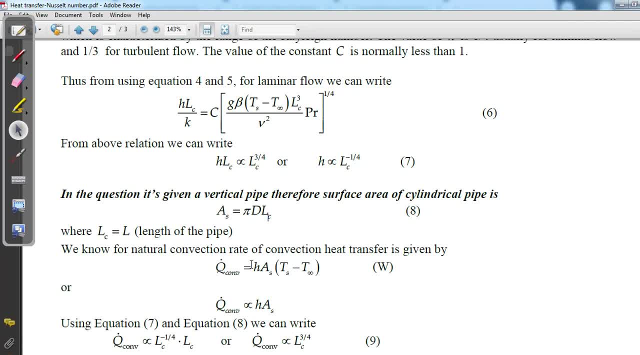 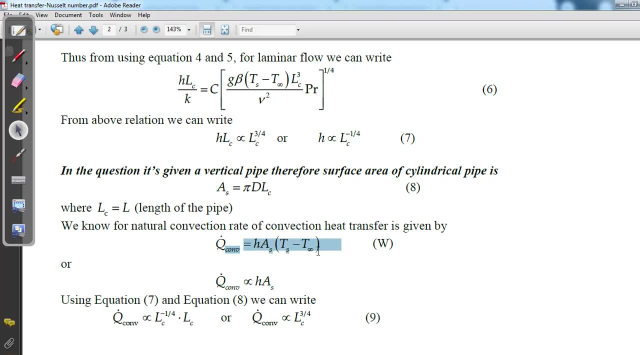 lc. lc is the length of the pipe in the given question. so from here we from that Newton's law of cooling. q convection is given as h as into t s minus t infinity. t s minus t infinity is constant. so we will remove from here and we will write that q convection is directly. 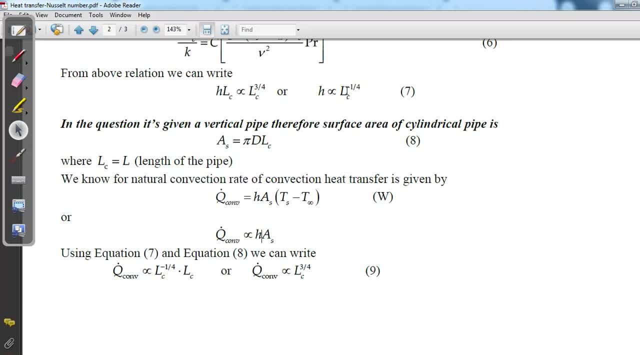 proportional to h into a s. h is directly proportional to lc, to the power minus 4, and area is directly proportional to- from this's video, this relation, because pi and d are constant, so it will a directly proportional to lc, so when this base will some and power will be get added, so minus 1 by 4 plus 1, so it will. 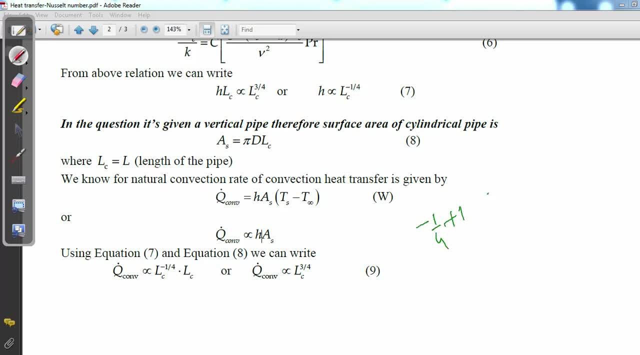 be minus 1 plus 4, divided by 4, equal to 3 by 4. ok, so q convection. this is the important formula we have to derive. so in most of the case in this equation we get q as q's. so q convection, skin convection. 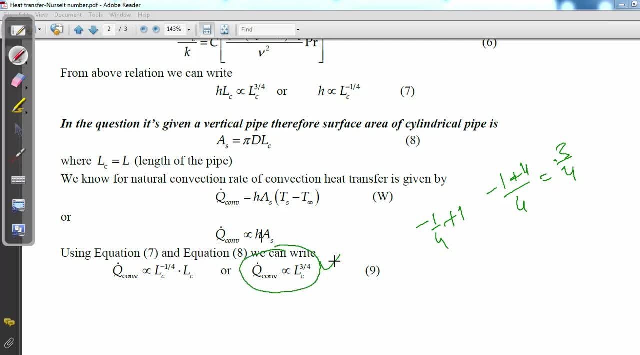 will be added. so in all solar regions we have to add qfen. so this is that: cn by cn. this is basically n 0 exactdy, half now the Gordonville in our solution of q. as this bulldon by a is the previous question, this formula is given directly, so you have to just mug up the question. 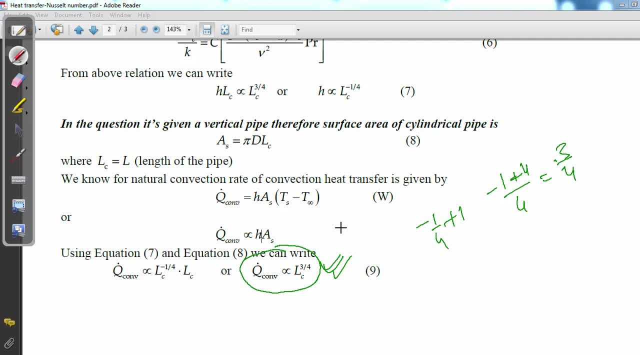 and you don't understand that how it is coming, because if the question will change, like for it is given for turbulent flow, then this value will change. so you have to remember this, okay, so what? what condition they are given for this? so we have arrived here, so now it's easy. we have. 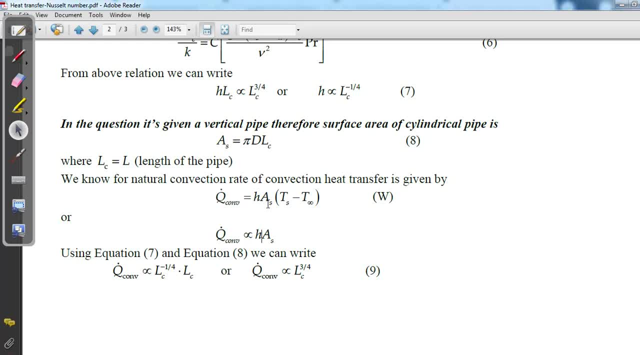 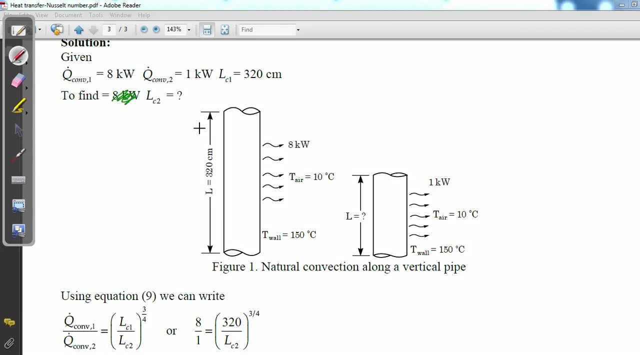 to just apply this formula and solve this question. so let's come back to the figure. and here it is saying that for first condition, 8 kilowatt Q convection is given Q convection 2. it is second condition. it is saying only 1 kilowatt for first condition. length of the pipe is 320 centimeter. 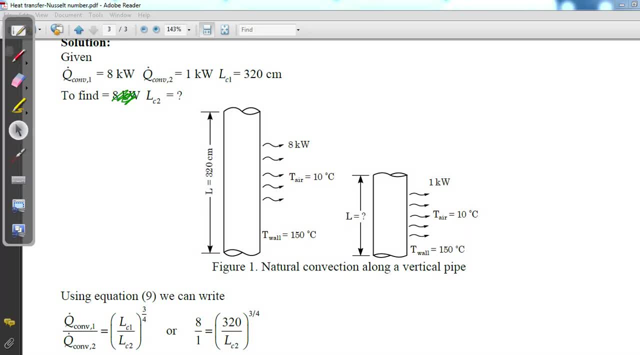 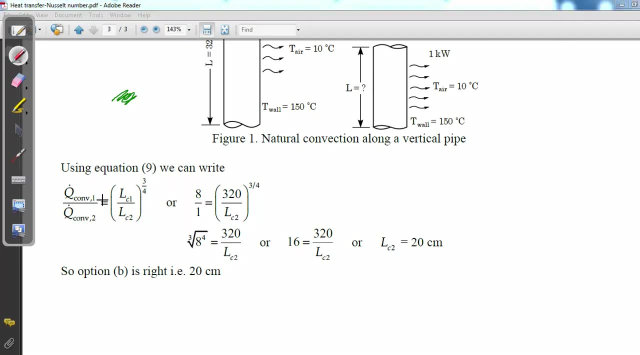 so we will put in this relation and we will solve further. so here it is given that Q convection upon Q convection 2, second first condition, divided by equal to LC2 to power 1, as it is directly proportional. so LC2 to power, LC1, condition 1, then LC2 whole to the power of.